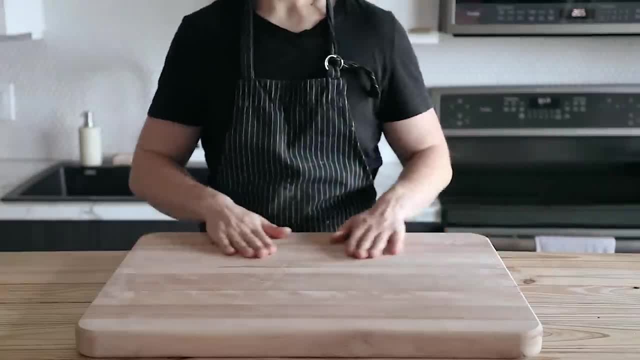 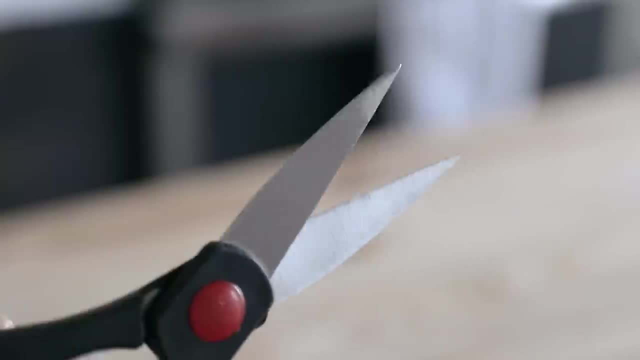 tasks than you would think other than just cutting stuff, and it's super economical if you don't want to buy a bunch of mechanical things like a food processor. Next thing is a personal favorite of mine, which is a pair of nice kitchen shears. These come in handy way more than you would think- Small. 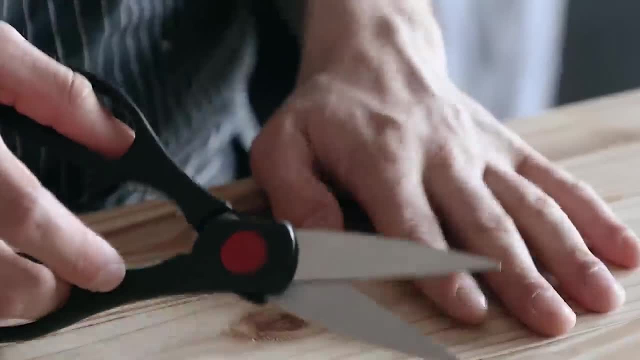 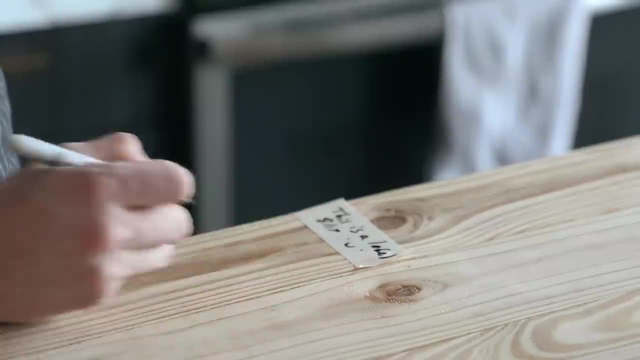 tasks like removing tough stocks from stuff without damaging your knife, cutting through small bones, and like chicken and fish. use something that you can get down and dirty with, Also in conjunction with that painter's tape and a sharpie, really great for labeling, so you can keep track of all your stuff Now. 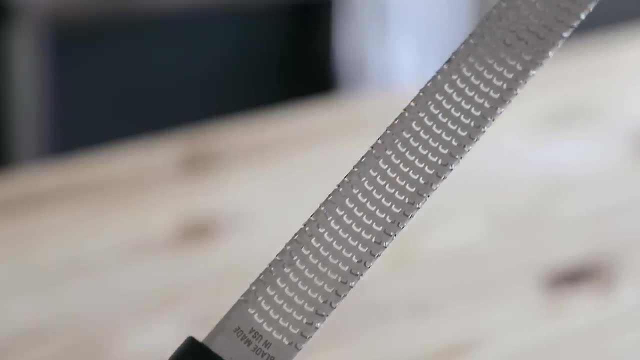 lots of people have a grater, but the one that I would really recommend is a microplane, which is really the best grater on the planet, If you want those nice delicate threads. you know I'm bougie. As for pots and pans, you know. 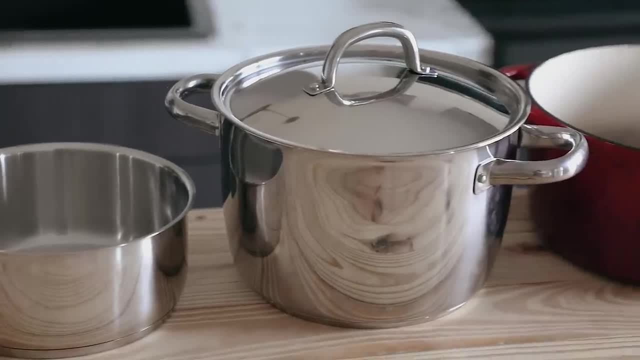 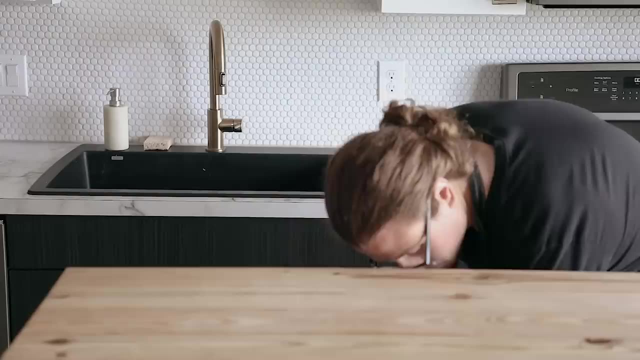 people really like to overcomplicate this. Just think about what you like to cook a lot, or the things that you might be cooking, and get the appropriate size. I have, you know, a small, medium and large of every style of pot and pan, because that's how I be. I would just recommend having 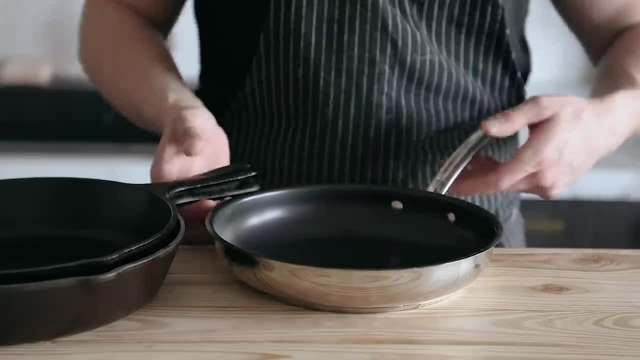 different kinds of surfaces. Have some that are nonstick, have some that are cast-iron. I'm a big fan of pans that you can put in the oven because they're multi-purpose and you can roast small amounts of stuff in them or finish a. 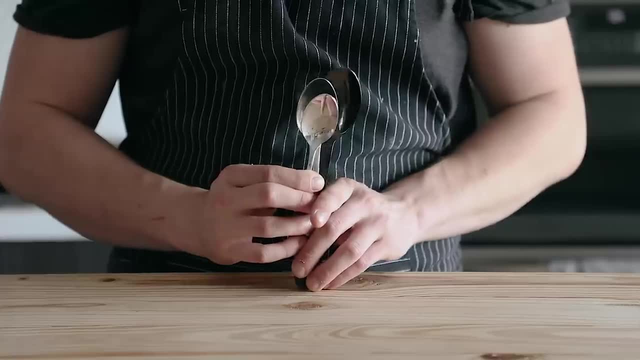 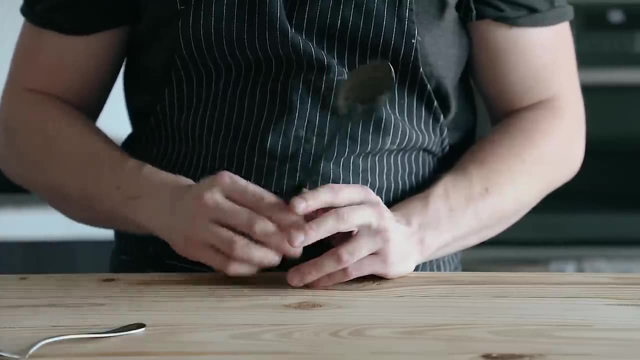 steak in the oven if they're heat-safe on the handle. Let's talk about spoons. You need different sized spoons: A because you can make more spooning puns, and B for multiple uses in cooking. Some will be for basting, some. 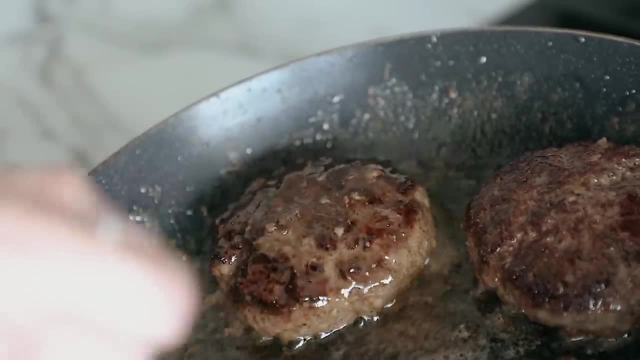 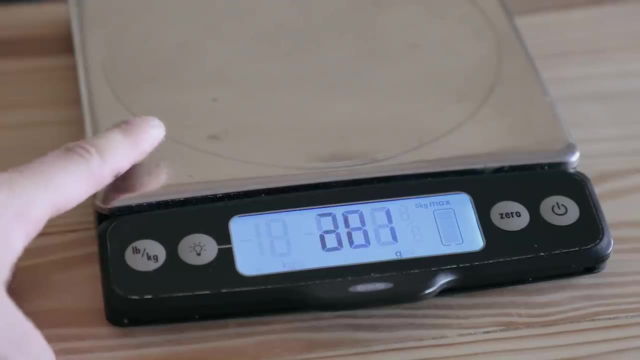 will be for sauce stirring, you know, efficient cereal eating. Just, you know the little things count. Sure, everybody has measuring spoons, but why not kitchen scales? I'm putting this on the necessity side because I want you to do my recipes in grams, Not shelf, not self, wow, not. 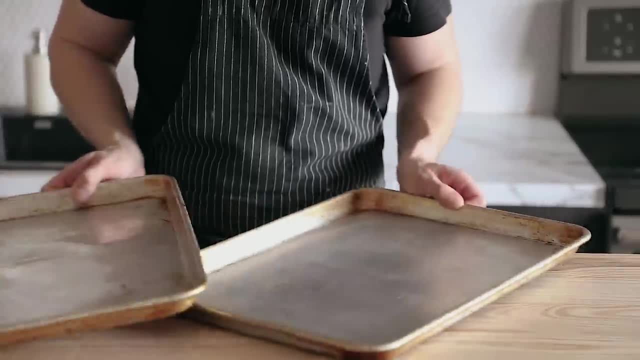 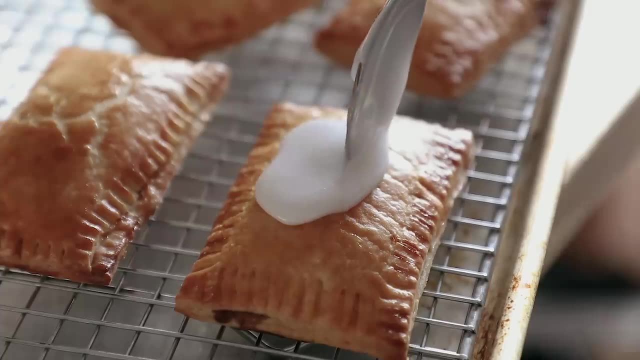 selfish at all. Baking trays and wire racks are the multi-purpose king of any kitchen. You can roast tons of things in them. use them for baking cookies. The wire racks can be used to drizzle chocolate over stuff or to ice donuts or. 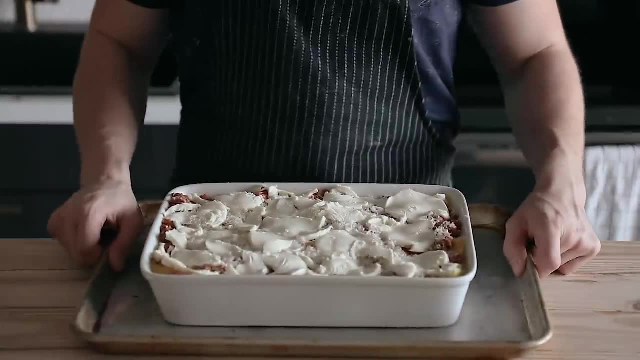 whatever, so that it falls beneath and it's easy to clean up. You know, there's just, there's just so many uses. Now, if you've known me long enough, you know that I'm a big fan of jars. These are like the storage love of my life. You. 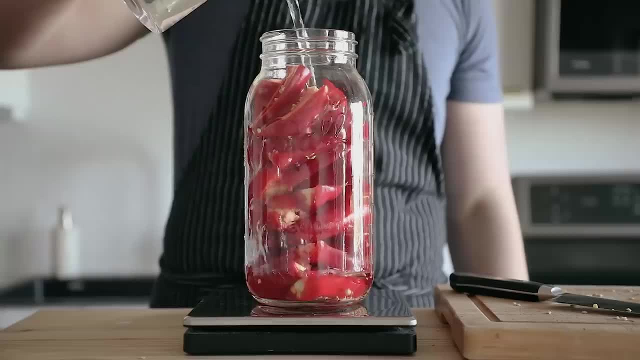 know, not only are they great for storage, but they're good for fermentation pickling. you know you can put sauces in them, oils- They're just, they're too good and they look so nice. I'm all about that jar aesthetic. you know what I'm. 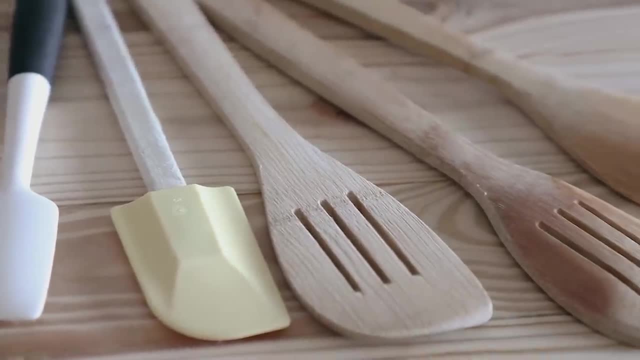 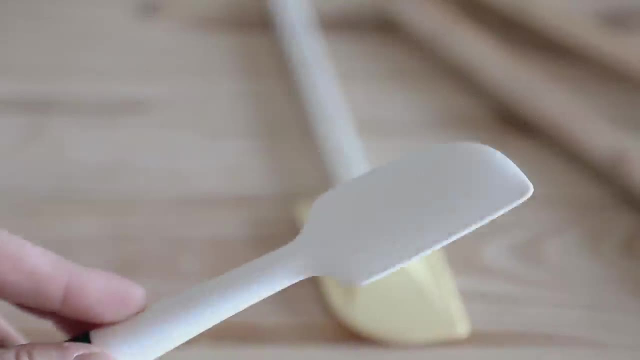 saying. Now, last but not least on the essential side, would be stirring spoons. I don't like to use metal stirring spoons. I much prefer to use something like a wooden stirring spoon or a silicone spatula, which are also great for scraping stuff out. The thing, the reason why I prefer wood, is just: you can. 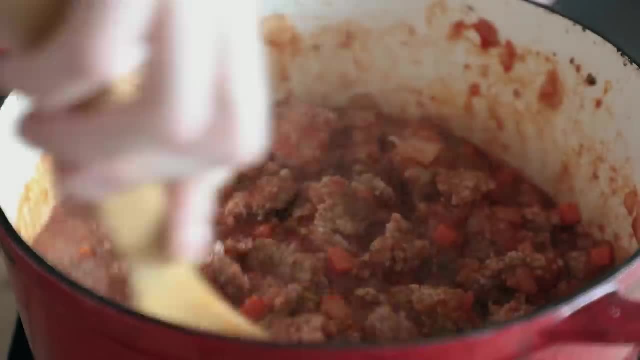 use them for pretty much any surface, because they don't scratch nonstick and they just look a whole lot nicer. Okay, so next piece is stuff that I prefer to have, but it's not a requirement Forewarning. this is the stuff that's. 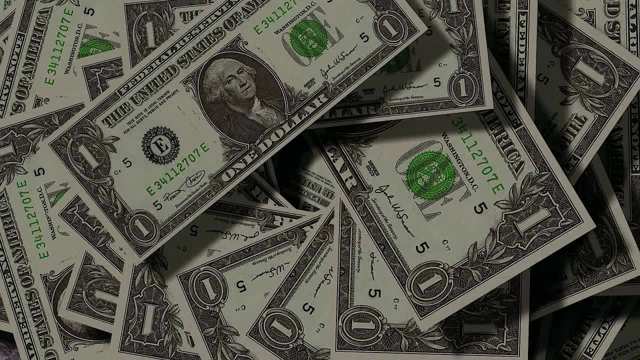 more expensive. so if anyone's like, oh my gosh, it's too expensive, these are not a necessity. You don't need to have a Lamborghini, but it's nice to have a Lamborghini, Alright. so number one on this list is the coveted KitchenAid. 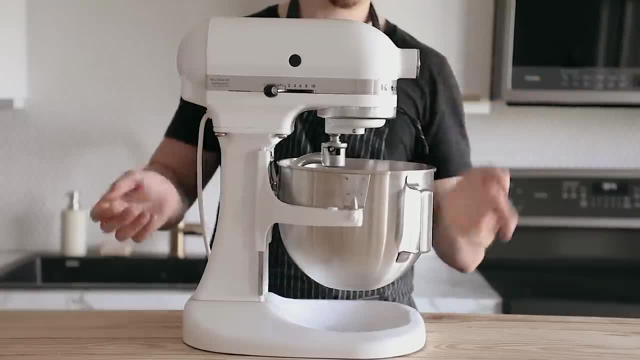 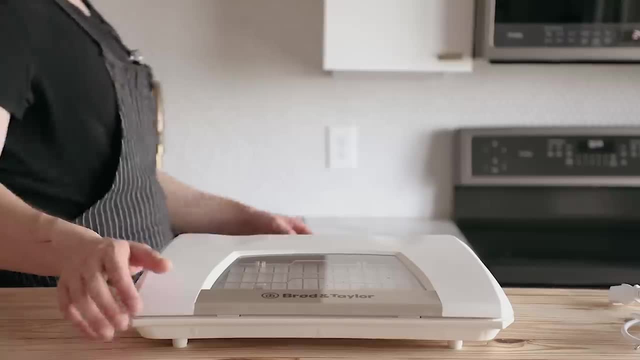 stand mixer, One of my most favorite tools in my kitchen. It does a million billion things other than just making dough. It does everything. I'm not even gonna try and sell you on this, It's too good. Next up on that is my fermentation. 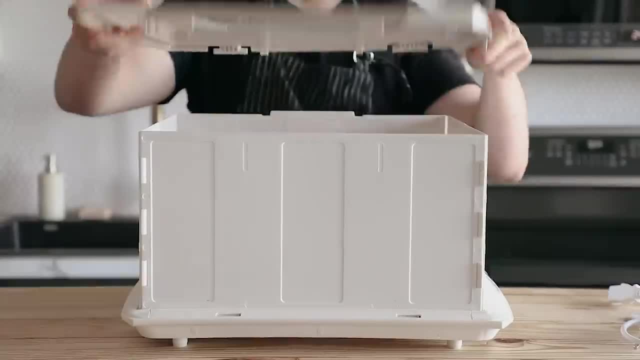 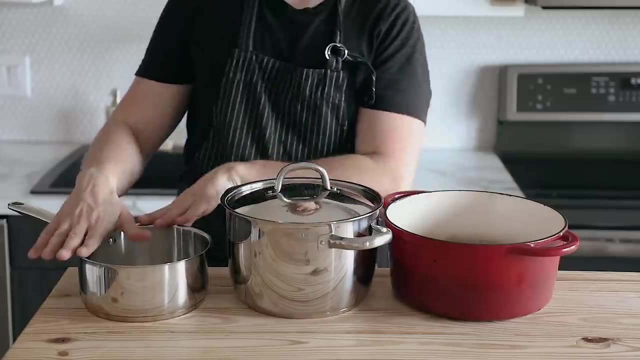 station. You guys already know how I feel about this thing too. I love this thing. It's great for making bread and fermentation. It is the perfect fermentation chamber. By the way, guys, just a reminder, all the links for this stuff is gonna be in the description if you want to see it, or? 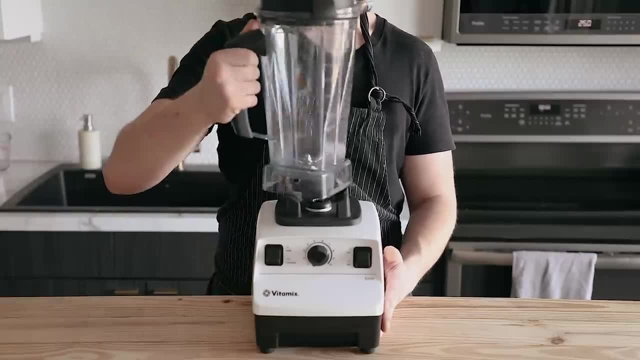 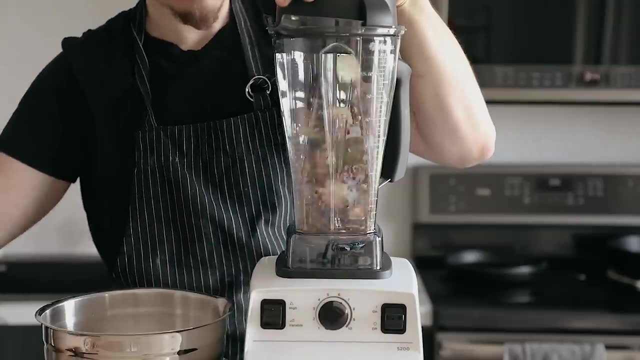 check it out. read about it. whatever Next up is gonna be a Vitamix blender. Now, I know these things are expensive, but this is an industry standard for a reason. You can blend and make anything so velvety smooth from nut butters to. 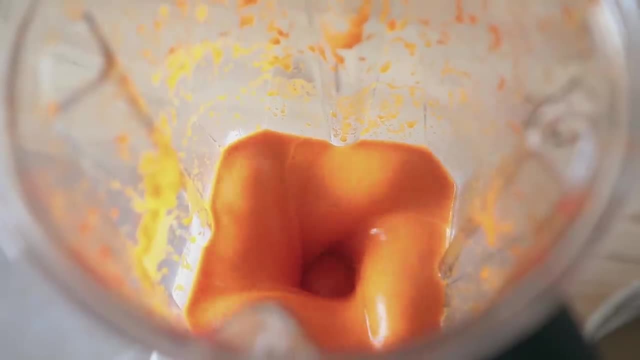 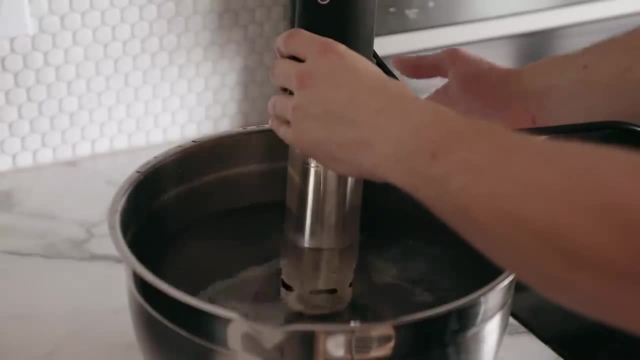 super useful. There's a couple different ones on the market, but there are two dominating brands that I really like and I'll have them linked below. It turns literally anything into a sous vide bath, so how can you complain about that? And 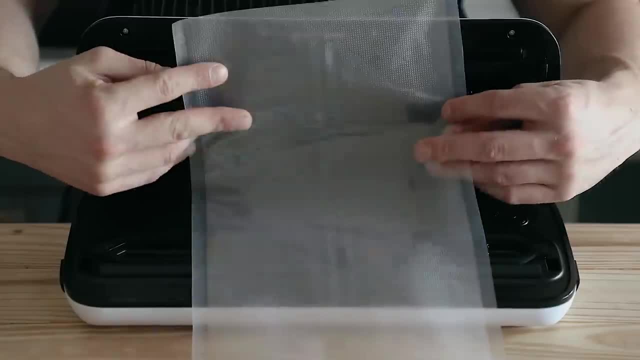 the last thing, which is also a follow-up to the sous vide circulator, is a vac machine and vac bags. These are obviously gonna be used for the sous vide. You vacuum seal your meats and then you sous vide them, but this can be used for so. 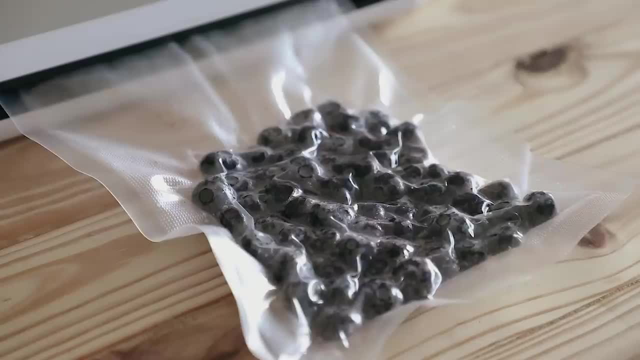 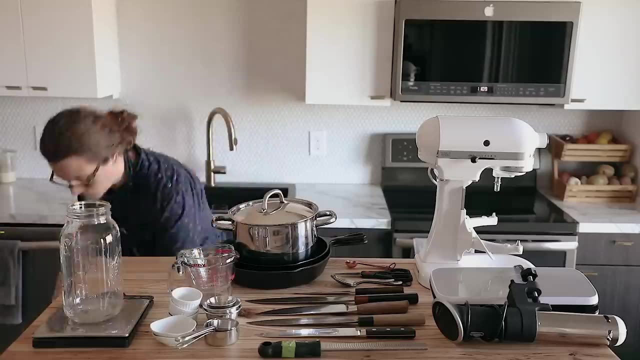 many things beyond that, Not just food storage, but you can use it to ferment things. I love to ferment berries with this. I'm fermenting some blueberries here and it just makes storage super duper efficient in your fridge or dry.